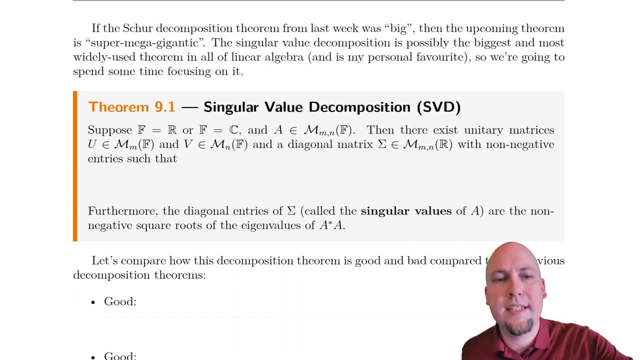 okay. So today's a big one, Let's get to it, okay. So what is the singular value decomposition? Well, as its name suggests, it's a decomposition theorem, and so what it says? well, it's kind of like diagonalization, It's kind of like the spectral decomposition. It says: okay. 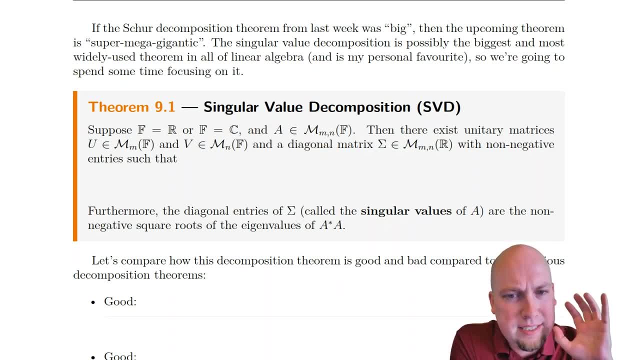 so if you've got some matrix here, well, they're going to exist Two unitary matrices, U and V, and there's going to exist a diagonal matrix such that you can decompose your matrix A, your original matrix. in this way, You can decompose any matrix. 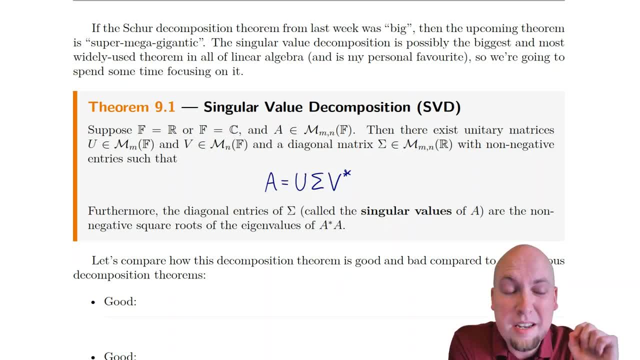 as unitary times, diagonal times, another unitary- okay, So this is very similar to other decompositions that we've already seen in this course, like the spectral decomposition, for example. So we're going to spend a while talking about how this is better in some situations, how it's different. 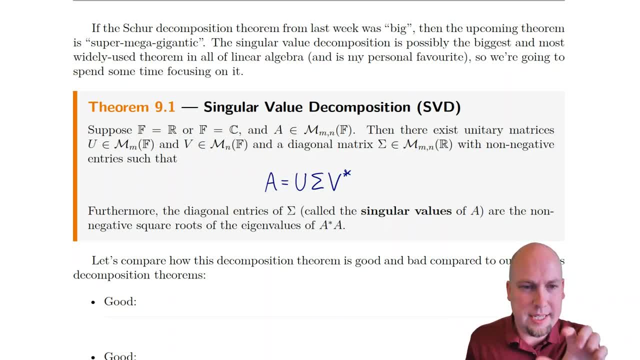 and sort of clarifying those points. okay, But there exists two unitaries and a diagonal matrix in the middle. Furthermore, the entries on the diagonal of this middle diagonal matrix sigma, here they're uniquely determined by A. okay, So we give them a name, We call them the singular. 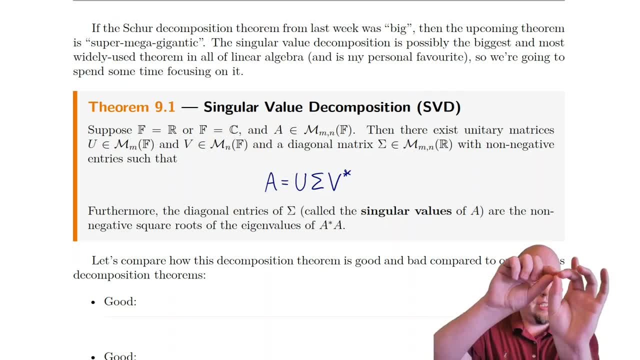 values of A. okay, Just like in diagonalization, the entries on the diagonal matrix D in the middle, those were the eigenvalues of A. Well, in the singular value decomposition, the diagonal entries in the middle diagonal matrix, we call those the singular values. okay, And they are. 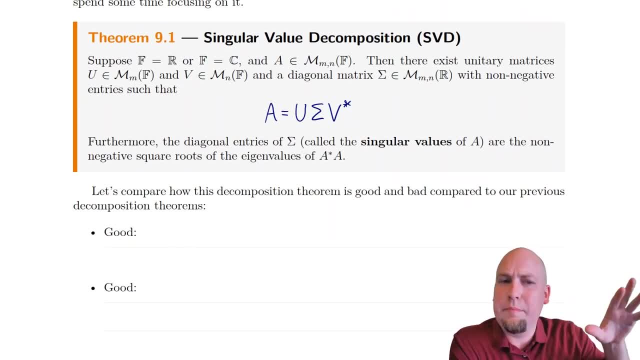 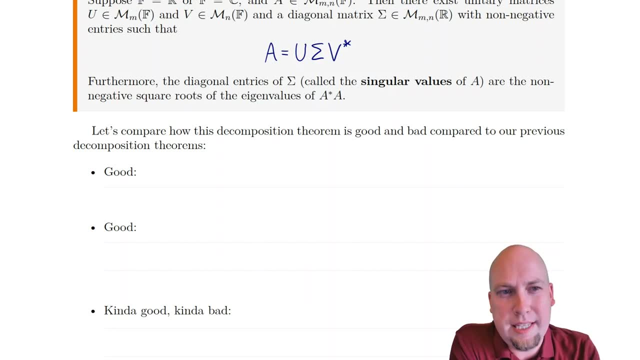 completely determined by A. Okay, so let's think a little bit about how this compares to other matrix decompositions that we've seen, okay, And how it's better than them in some ways and it's worse than them in some ways. Mostly better, though, okay. So one thing that's good. 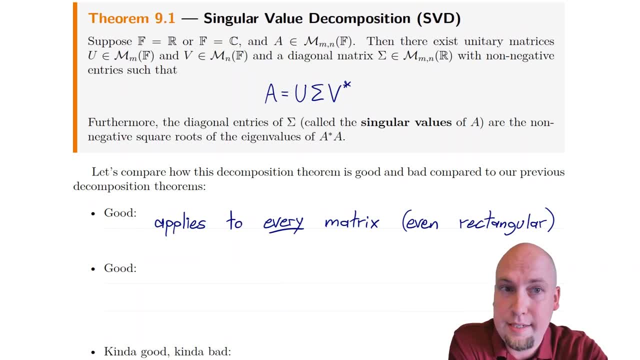 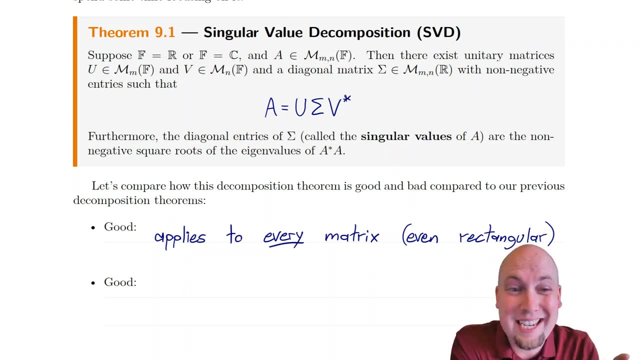 about this decomposition. one thing that's really nice and better than any decomposition theorem that we've seen so far is this theorem, the SVD. it applies to every single matrix, even rectangular matrices. right Here A, it can be M by N. No other decomposition that we've 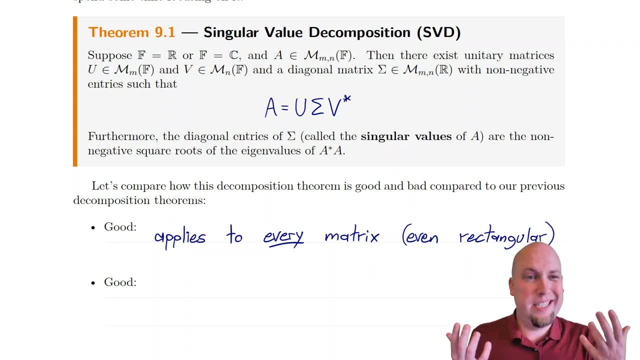 looked at has been like that: right, Regular diagonalization needs to be square matrix. Sure, triangularization needs to be a square matrix. Spectral decomposition needs to be a square matrix, and even normal, okay. So here we've got a leg up, okay? It applies to every. 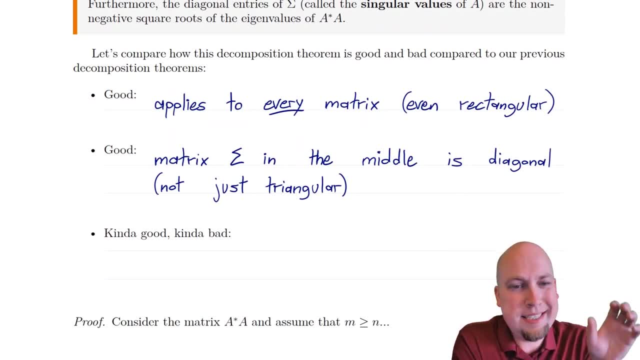 matrix. Another thing that's nice about this theorem is that sigma in the middle it really is diagonal. It's not just upper triangular right. I mean, like when we have a decomposition theorem that works for so many matrices, maybe our mind goes back to sure triangularization. 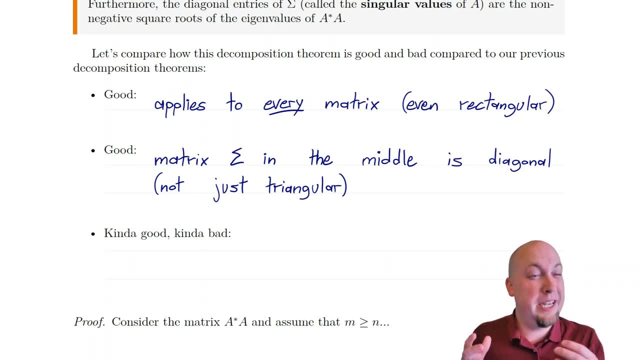 right. That worked for any square, complex matrix, But here we've got a leg up over that. We get a diagonal matrix in the middle, not just an upper triangular one, And furthermore that diagonal matrix in the middle- it's always real, even if the matrix A itself is complex, And furthermore the diagonal entries. 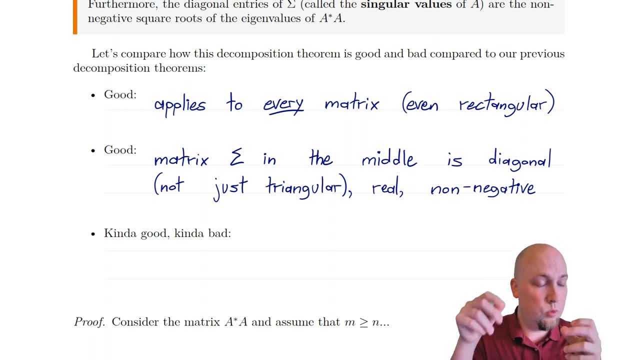 on that diagonal matrix. they're non-negative, okay, They're real and bigger than or equal to zero. We haven't had any decomposition theorem like that yet. right, The spectral decomposition and regular diagonalization. you just had eigenvalues in the middle, And even for real. 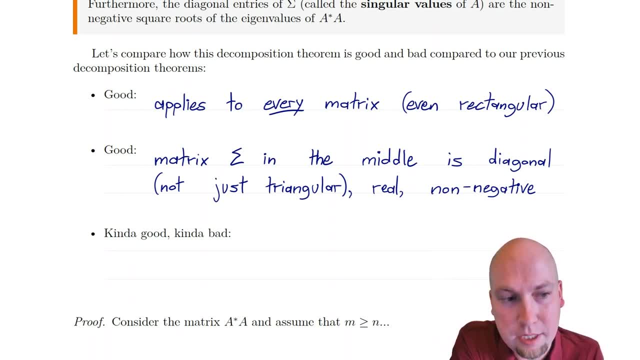 complex eigenvalues, so a complex matrix in the middle of diagonalization. But that doesn't happen here. Here we always get real non-negative matrix in the middle, real non-negative diagonal matrix- Okay. but the trade-off for getting these nice features is that now you 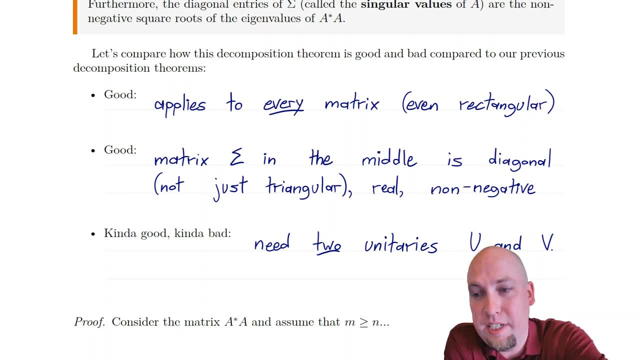 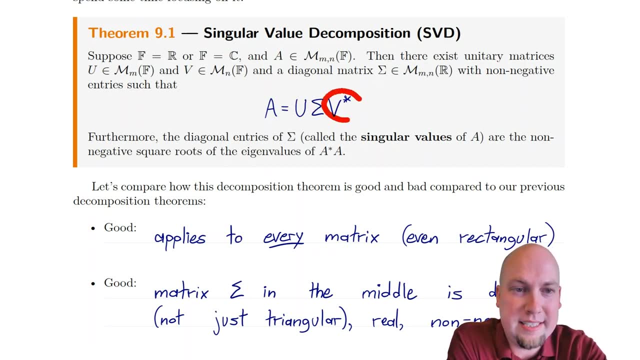 need two unitary matrices, U and V right. We have a different unitary on the left and on the right in this matrix decomposition right. In the previous decompositions we always had you know something over here and then it's inverse on this other side. 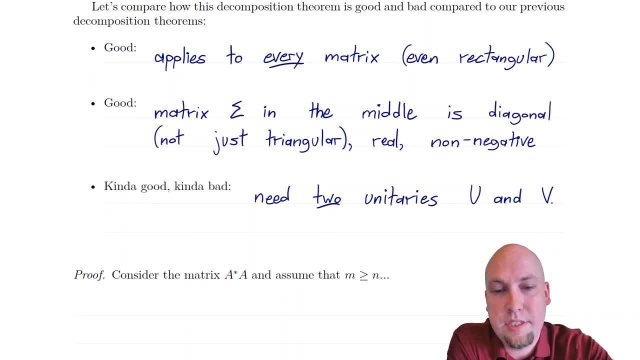 whereas that's not the case here. We have two potentially different unitary matrices. Okay, but on the flip side, you know, it's kind of good, kind of bad. It's worse than having just one unitary matrix, but maybe it's better than having an invertible matrix like in regular 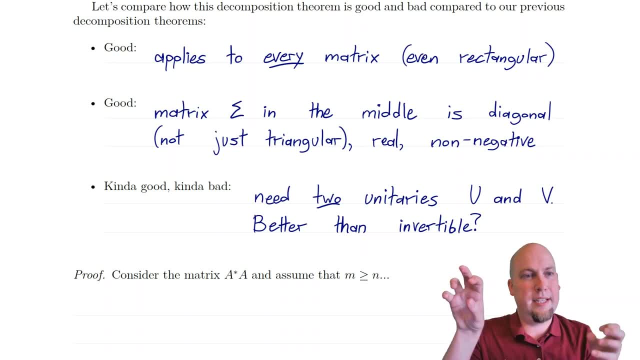 diagonalization, right Diagonalization, you have invertible matrix P then D, then P, inverse. Maybe two unitaries are nicer than one invertible. I don't know. There's some sort of trade-off there. All right, so let's prove this theorem. Unfortunately, we've actually done all of the 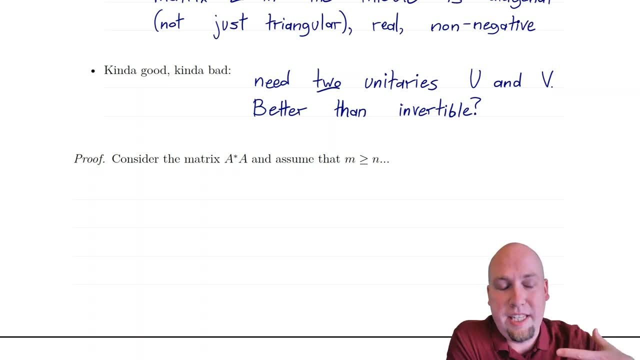 heavy lifting already. We're just going to leech off of theorems that we've been seeing and developing over the last few weeks, couple weeks, okay. so the way that we're going to prove the singular value decomposition is: we're going to consider this matrix, we're going to consider a star a and we're going to get the 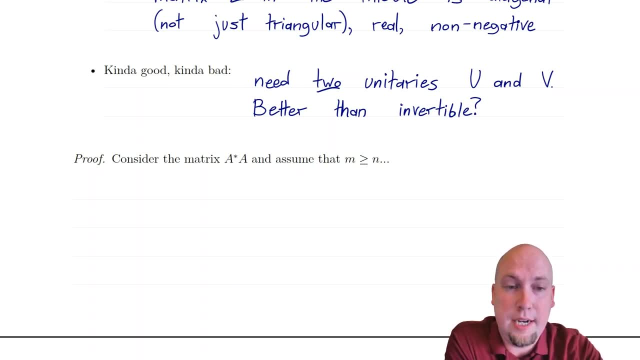 decomposition for a itself out of some decomposition for a star, a. okay, but this is assuming that m is bigger than or equal to n. on the other hand, if m is less than n, in other words, if you have fewer rows than columns, you're going to want to use a a star instead. okay, and you'll be able to mimic. 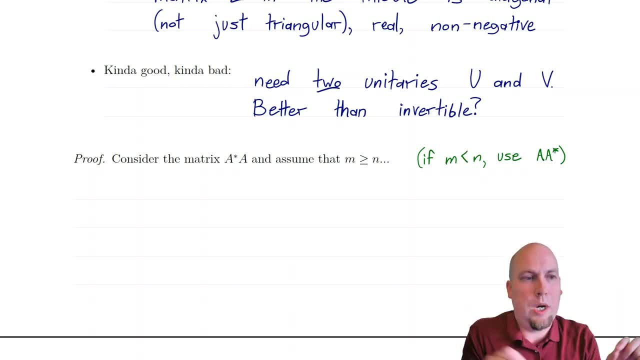 everything else that we do in this proof. you just make that sort of swap there and you'll get. things will sort of change accordingly all the way through, but you still get the same decomposition at the end of the day. okay, so here's the argument. a star, a well, we know that's positive. 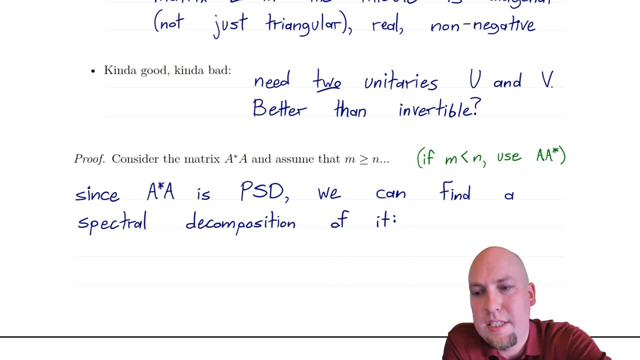 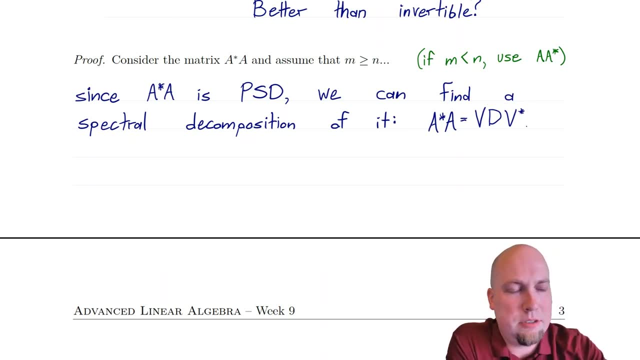 semi-definite. that's the form of a positive semi-definite matrix, right? so we can find a spectral decomposition of it. so let's just write that down. okay, a star a: it's positive semi-definite. so here i've just written down some spectral decomposition of it. so d is diagonal and v is. 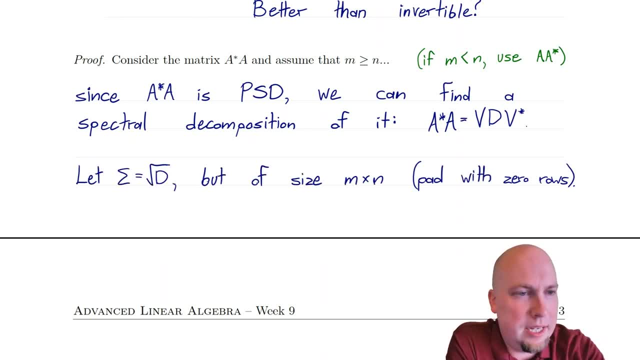 unitary, and because a star a is positive semi-definite, we know that actually the diagonal entry is a positive semi-definite, so we know that a star a is a positive semi-definite, so we know that a v, star f of d are real and bigger than or equal to zero as well. okay, so in particular, 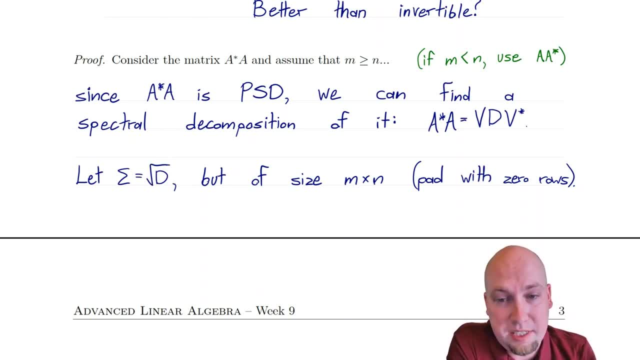 we can take square roots of them and we'll get real bigger than or equal to zero things along the diagonal of this matrix, root d, okay. so what i'm going to do is i'm going to say, okay, well, let's sigma, the sigma part of the svd, let it be this root d matrix, except i'm going to be careful. 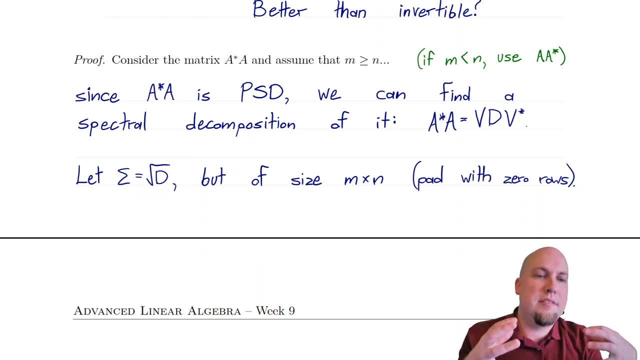 i'm going to pad this matrix sigma so that it's not of size m by m, or, sorry, it's not of size n by n, but rather a size of size m by n, right, okay? so we're assuming that n is the smaller one here, and if you go through and check the size of these, 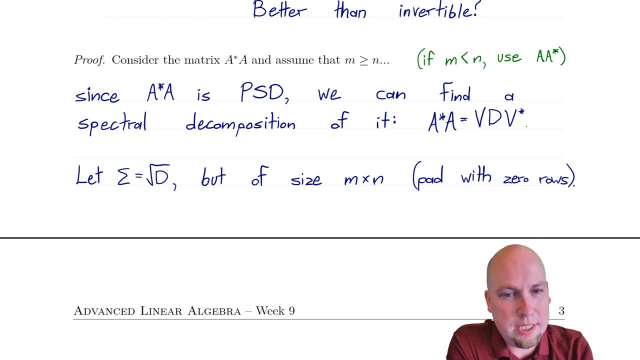 matrices d is going to be an n by n matrix. So when you take square root of it it's still an n by n matrix, and we're just going to add on some extra zero rows to make it m by n instead. So that's a fine thing to do, fine and dandy. So now we've got an idea of what the v part. 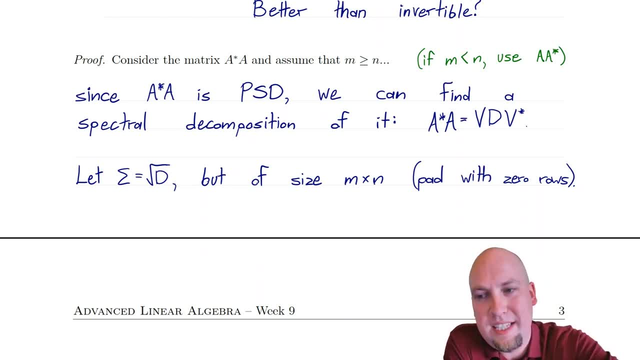 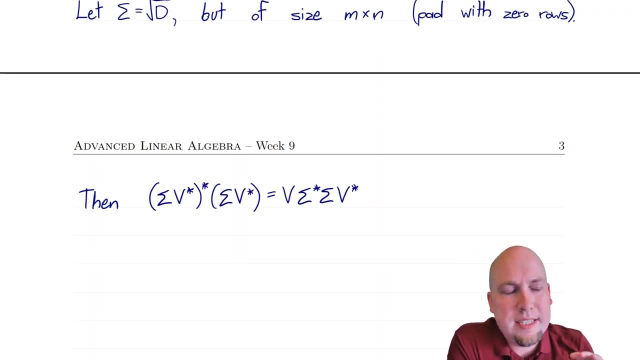 in the singular value decomposition is going to be, and we've got a feeling for what the sigma part in the singular value decomposition is going to be. We just need to construct u now. So where does this come from? Well, this comes from that sort of helper theorem that we saw last week. 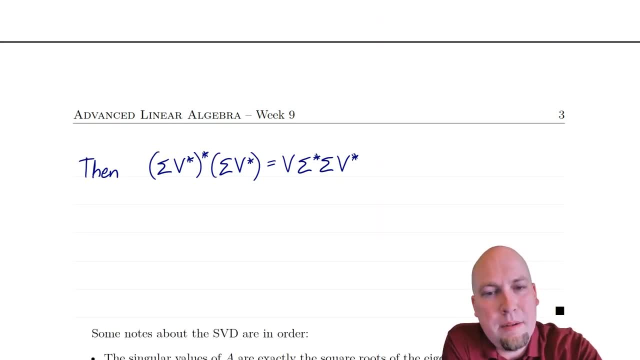 What I'm going to do is I'm going to compute what I get if I multiply sigma v star by its own conjugate transpose, Just using standard rules of matrix multiplication, all of our usual theorems here. I mean, we have a star on a bracketed term, so just apply it to both and 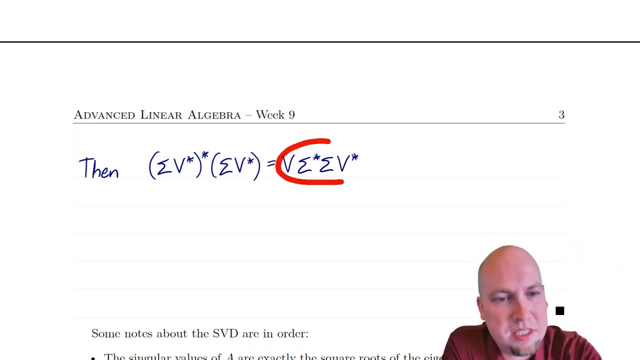 flip the order of the multiplication there. So you're going to get v sigma star, sigma v star. When I do that, okay, and remember where? what is sigma? Well, sigma is the square root of d, so you have to be a little bit careful with the sizes of these matrices, right? 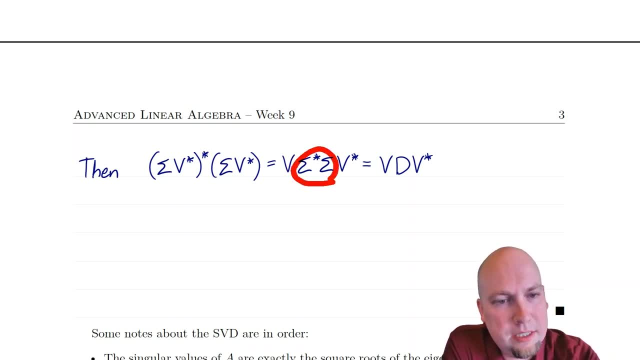 Sigma is m by n. so when you do this product here, you get an n by n matrix, which is exactly what d is. okay, Everything works out. You get the n by n matrix d on the middle here when you multiply these guys together. All right, so we get v d v star. but wait, what's v d v star? I've. 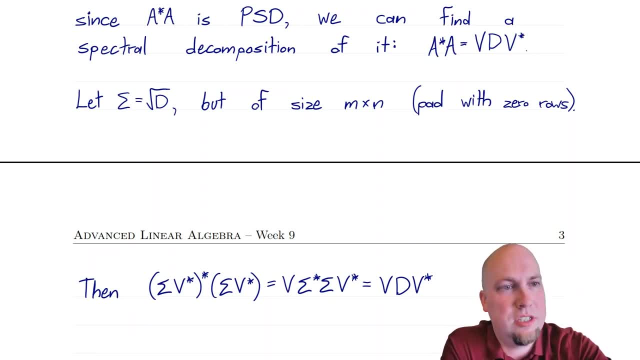 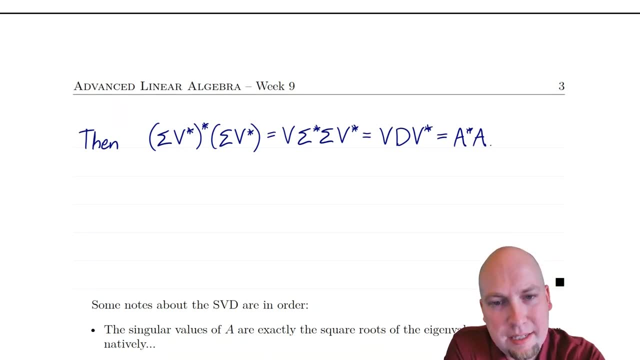 seen that. Ah, that's exactly the spectral decomposition of a star a that I started with up and down. So that's exactly the spectral decomposition of a star a that I started with up and down There. okay, so that's a star a. Now I'm going to look at what I got here. I've got something. 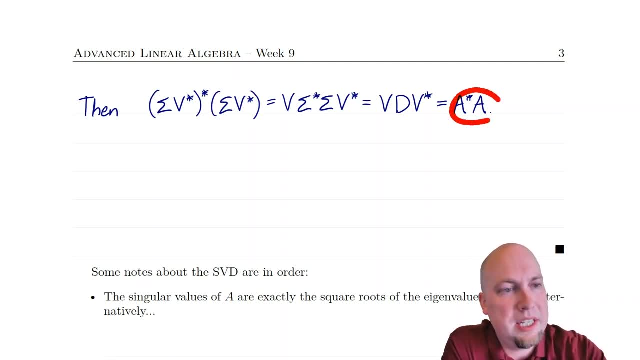 something times its own conjugate transpose equals something times its own conjugate transpose. We have a theorem from last week. Theorem 8.7 tells us exactly when that happens. right, This was the theorem about how can you have two different decompositions of a positive. 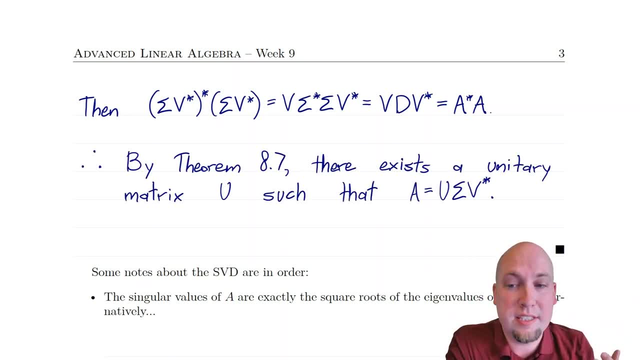 semi-definite matrix. Well, if, and only if, there's a unitary matrix that relates them. If, and only if, there's a unitary matrix such that this guy equals unitary times this guy. So there is exists some unitary matrix u such that a equals u sigma v star. And that's exactly what we wanted. 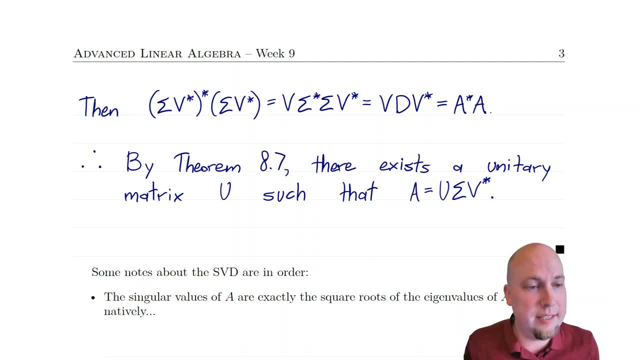 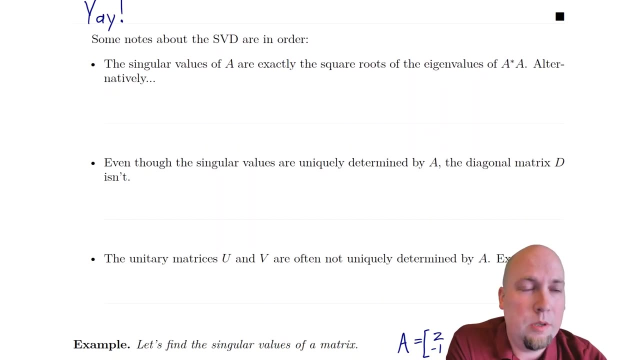 Now we have the entire singular value decomposition just sitting there right staring at us in the face. Okay, so that's it. Now we're done. the the proof of the theorem. So, yay, we're happy. Okay, that's it All. right. so there are a bunch of notes that we want to make about this theorem before we get. 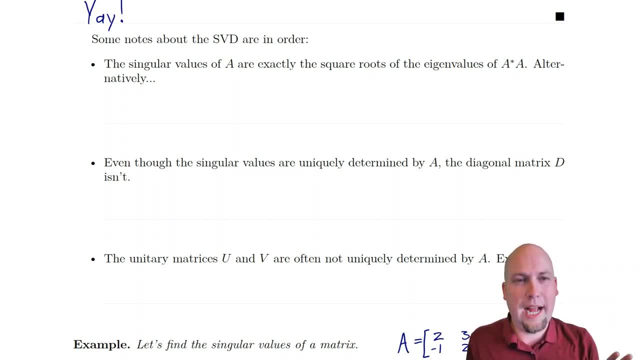 around to, you know, actually computing and all that sort of stuff. Okay, so how would we compute this in practice? Well, if we sort of trace through the proof up above, we notice that, hey, the singular values of a, the entries on the diagonal matrix sigma, they're the square roots of the eigenvalues of a star, a. 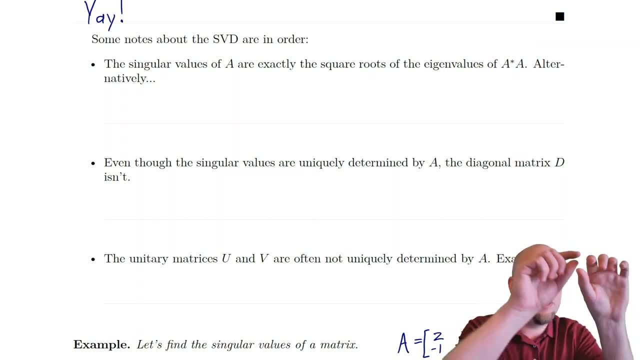 right. What we did was we did a spectral decomposition of a star a and then we took square roots of the d part, So we took the square roots of the eigenvalues of a star a. Okay. alternatively, equivalently, if you go through the proof with a, a star instead of a star a. 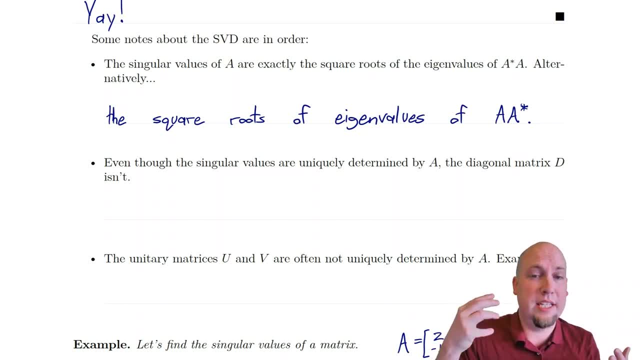 you get the exact same thing. The same decomposition pops out. So a corollary of this is that a star, a and a a star, they have the exact same eigenvalues of each as each other. So it doesn't matter which of these two matrices you use to find the singular values. 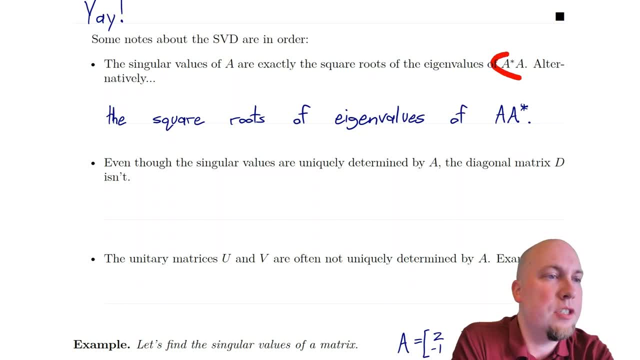 of a itself. Okay, with one slight caveat: these two matrices, they might have different sizes. Okay, so they have the same non-zero singular values actually, or sorry, the same non-zero eigenvalues, except whichever one's larger is going to have some extra zero eigenvalues tacked on. 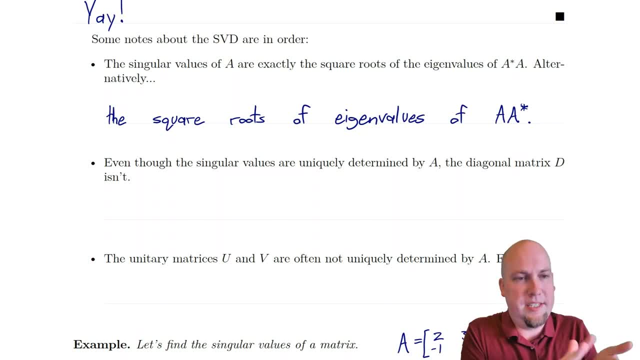 Okay, so they have the same eigenvalues up to you know however many zeros. Okay, it's also worth noting how unique and non-unique the pieces of the singular value decomposition are. Okay, so that middle diagonal matrix sigma, even though the values along the diagonal, the singular values of the original matrix a, even though those are uniquely determined, 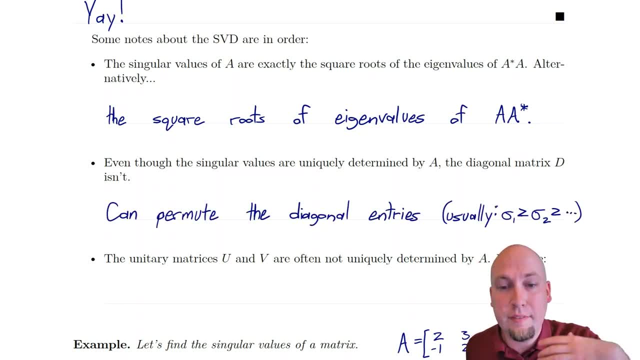 by a. the diagonal matrix sigma itself isn't Okay. you have a little bit of a little bit of freedom there in how you construct sigma. In particular, you can arrange those singular values in any order you like You can find a singular value. decomposition of your matrix a. 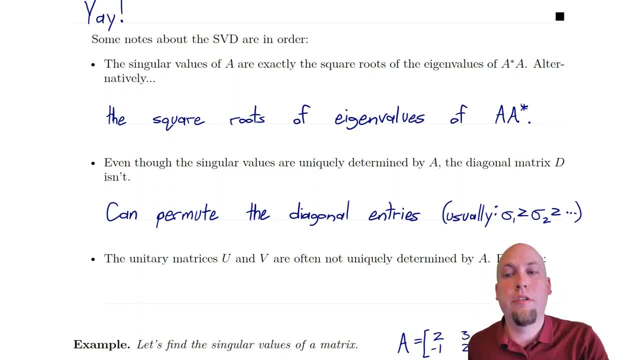 that has them in whatever order you choose. Okay, so usually, just for the sake of convention and pinning down a particular singular value decomposition, we usually order the singular values so that you know the largest one is what we call sigma one. it's the top left entry. 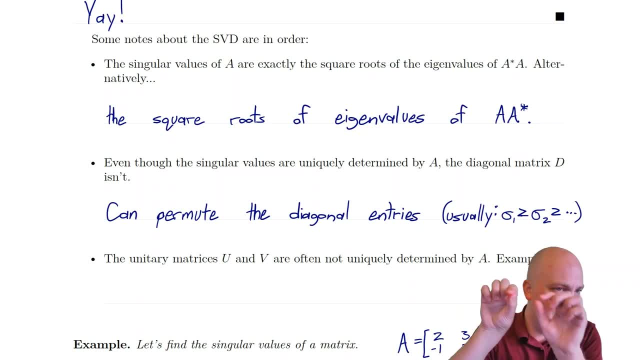 The second largest singular value is sigma two. the second, the, you know, the two, two entry in in the matrix sigma, and so on down the line, down to the smallest ones being at the bottom right corner. Okay, but even once you take that into account, even once you fix a particular ordering, 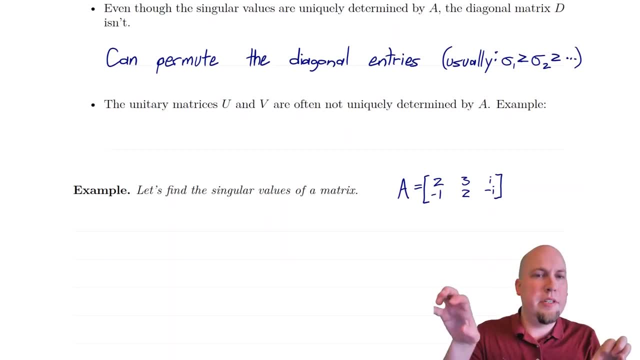 of the singular value decomposition, you're going to find that the singular values along the diagonal of that middle diagonal matrix, you still have these unitary matrices u and v, and those are often not uniquely determined by a. well, they're never uniquely determined by a, but sometimes. 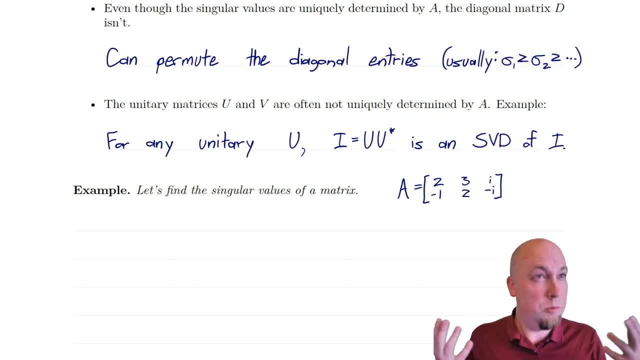 there's lots of flexibility in how you can construct them, Okay. so, for example, if you ask yourself, well, what are the singular value decompositions of the identity matrix? Okay, well, there's a whole boatload of them. in particular, you can pick any unitary matrix u. 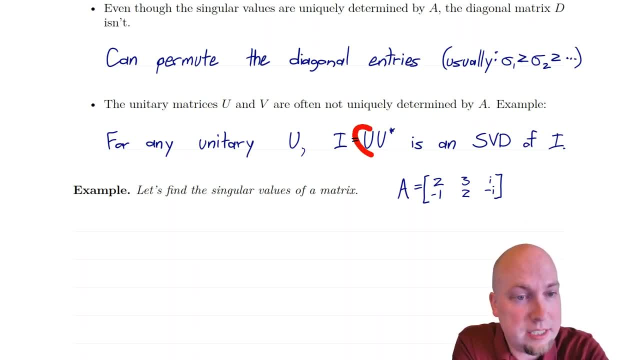 then u times u star is a valid singular value. decomposition of the identity matrix Right. here's my unitary on the left, here's my unitary on the right. and then there's just an identity. a diagonal matrix sigma equals the identity in the middle. Okay, so we can pick any unitary matrix that we 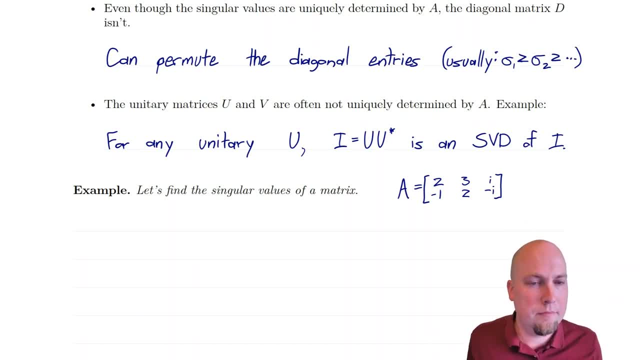 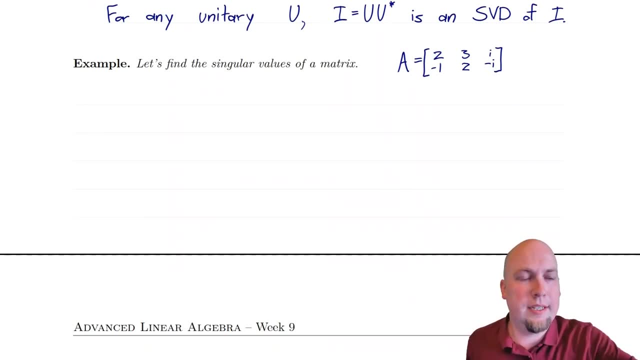 like, and then you just pick v to be the same thing. Okay so singular value decompositions. at least you know the unitaries, those in general. you know they're not unique. okay, All right, let's go through. let's actually compute the singular values of a matrix. we'll go through. 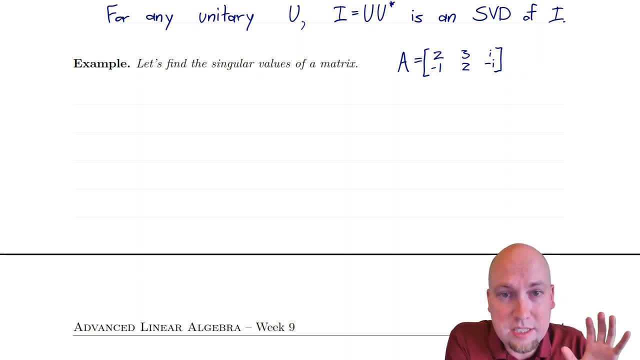 finding a full singular value decomposition in a minute, but for now let's just talk about how to find the singular values. we already talked about how to do it. let's do it, I guess. Okay, and the answer is: well, just as with most of these matrix decomposition theorems, 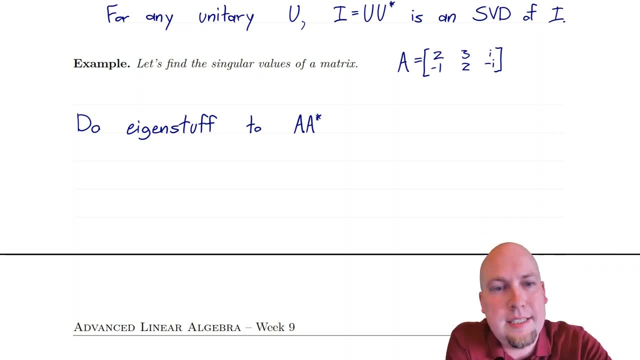 the answer is: do eigen stuff. okay, and this time we're doing eigen stuff to a, a star. we could do it to a star a, but I'm gonna do it to a, a star, and I'll talk about y in a second. Okay, so, first off, compute a a star, all right. so there's a, there's a star. 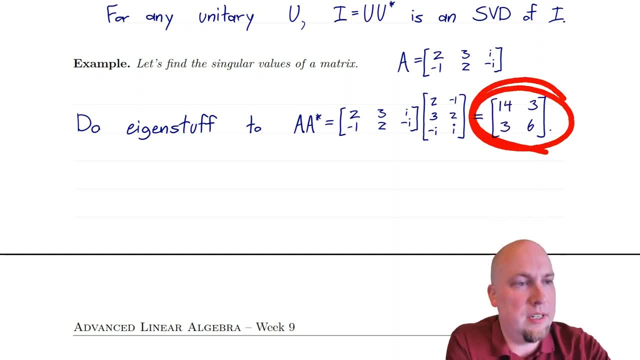 conjugate transpose and I multiply them together and I get this matrix here: 14, 3, 3, 6.. Okay, you'd something positive semi-definite. okay, so that is positive semi-definite, we're happy. okay, if you get something that's not positive semi-definite, you did something wrong. 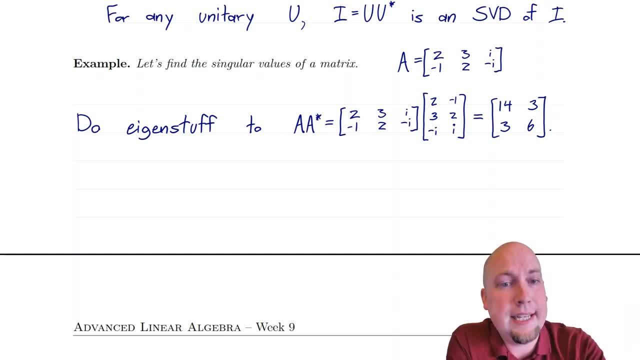 All right now notice that this is a two by two matrix. the reason that I used a a star instead of a star a is if I used a star a, I would have gotten a three by three matrix okay, and so computing eigenvalues of that three by three matrix is more work than computing eigenvalues of. 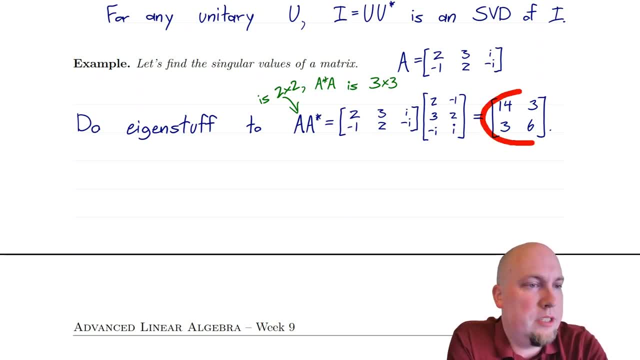 this two by two matrix. Okay, so I like working with the two by two matrix a little bit better, because it makes my computations easier. to do a star a. it's going to have the exact same eigenvalues as this matrix, except also an extra zero eigenvalue. that's the only difference. 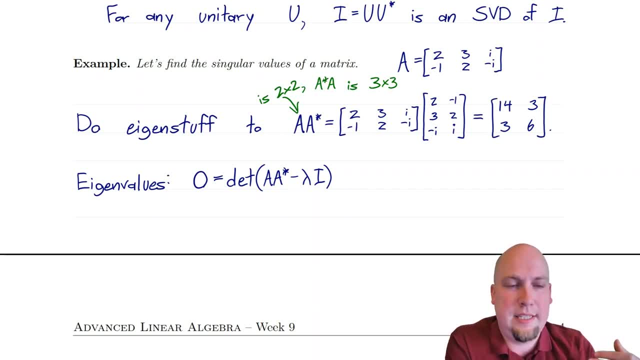 All right. so next up, we have to find the eigenvalues of this matrix and then, at the end of the day, we're going to square root those and that'll get me the singular values of the original matrix, a. All right, so set the characteristic polynomial of a a star equal. 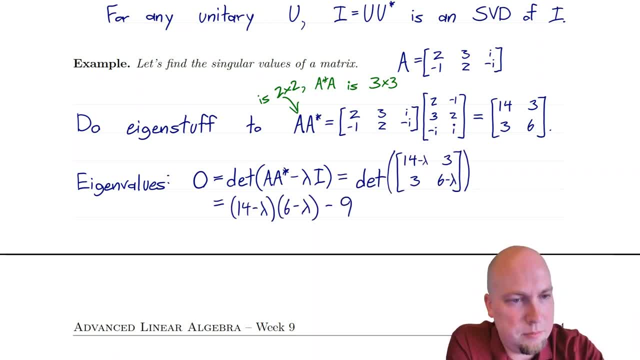 to zero. so subtract line is off the diagonal. take the determinant, all that jazz. okay. so product of the forward diagonal Minus product of the backward diagonal. and now I just expand that out, I get lambda squared minus 20, lambda plus 75. okay, so that's my characteristic polynomial, that I'm saying equal to zero. so I find 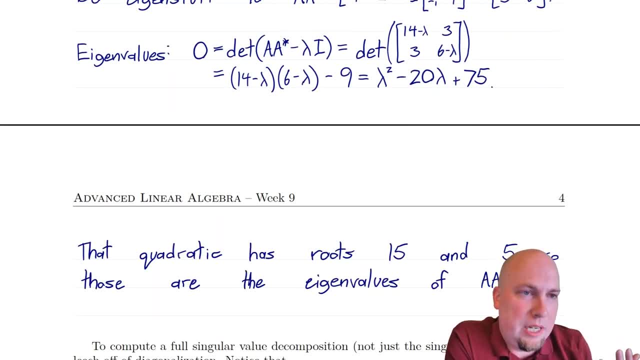 roots of that. okay. well, it's a quadratic equation. I know how to find roots. okay, it turns out this one: you can factor. but even if you don't see the factorization, you can just use the quadratic formula. and it turns out that the eigenvalues, the roots of this polynomial, are 15 and 5. okay, 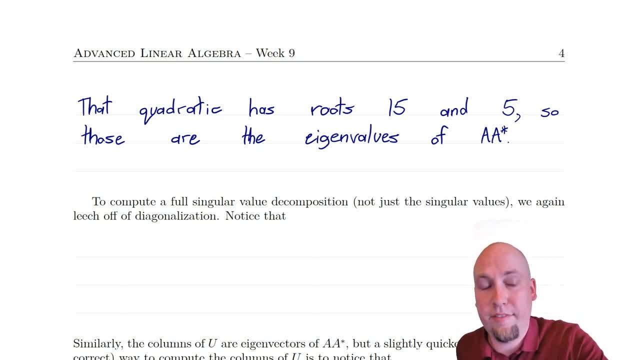 so those are the eigenvalues of a, a star. okay, so how do you find the singular values of a itself? okay, so let's square root those. okay, you get. so my largest singular value, what we'll call sigma 1, is root 15, and my second largest singular value, which we call sigma 2, that's root 5.. 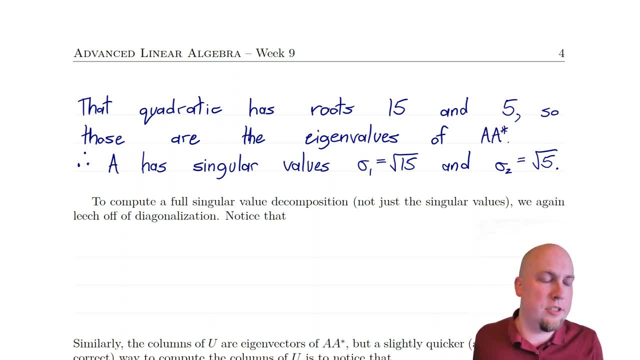 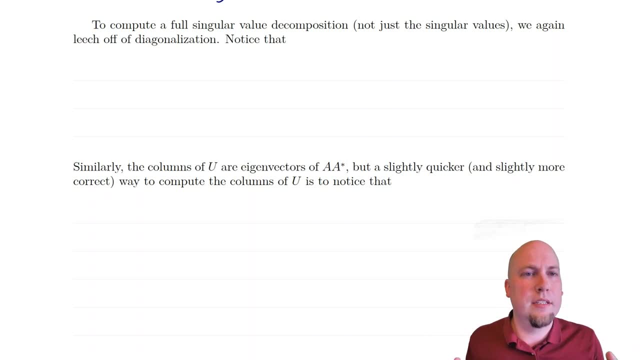 All right. so that's all there is to it. it's just your usual eigenstuff calculations, just with a square root thrown on at the end of the day, all right. well, how would we ramp this up if we want to find a complete singular value decomposition, so not just the sigma matrix in? 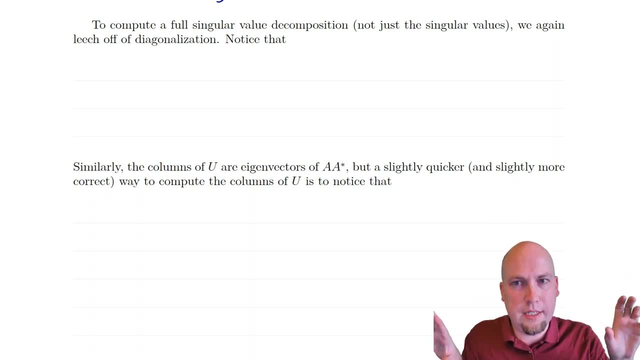 the middle, but also the u and v unitary matrices on the left and right. okay, so again, we're going to leech off of diagonal and we're going to find a square root of sigma 1.. Okay, so what we're going to notice is that, hey, if I've got some singular value. decomposition of a. 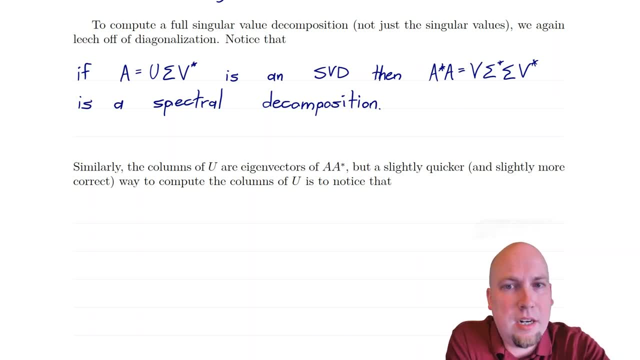 then, well, what do we have of a star a? well, a star a. if you just plug this in and simplify things a little bit, you're going to get v sigma star, sigma v star. okay, and what is this? well, it's a spectral decomposition. right, here's a unitary. here's the conjugate transpose of that same. 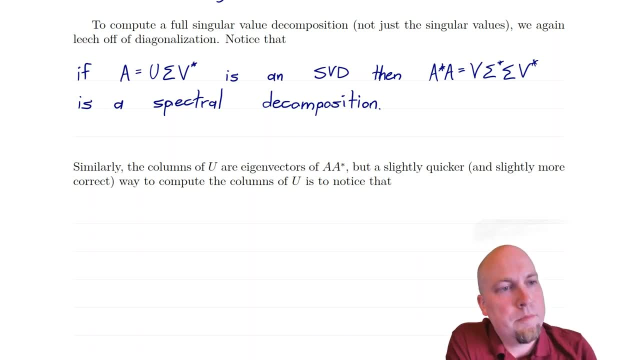 unitary, and in the middle we got some diagonal matrix. okay, so this is exactly what we're going to have: a spectral decomposition of this matrix, a star, a- okay. well, how do you construct a spectral decomposition? well, in the center. here, these are going to be eigenvalues. we already knew that. 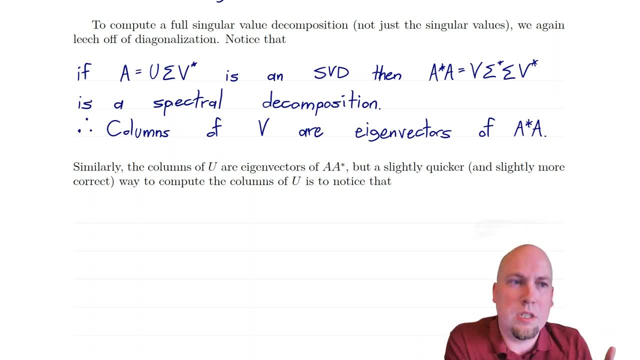 and the unitary matrix on the sides, while its columns are corresponding eigenvectors. all right, so the way that you can construct this unitary matrix v is you construct the corresponding eigenvectors from a star, a, okay, corresponding to the eigenvalues that give you the singular values. 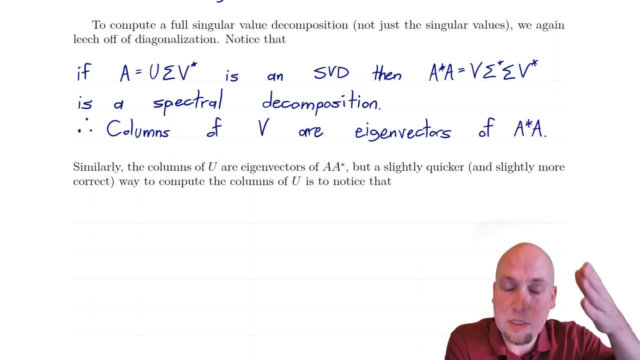 of a. okay, so eigenvectors are just eigenvectors that are on the side of the set. So let's start with a. vectors of a star, a, those give you the columns of the unitary matrix v. all right, similarly, you can do a similar sort of argument to show that the eigenvectors of a, a star, now those give you the. 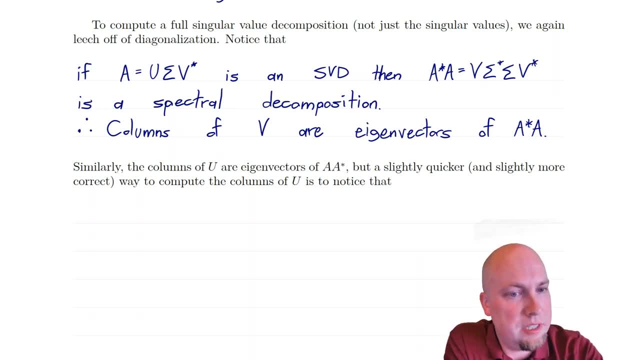 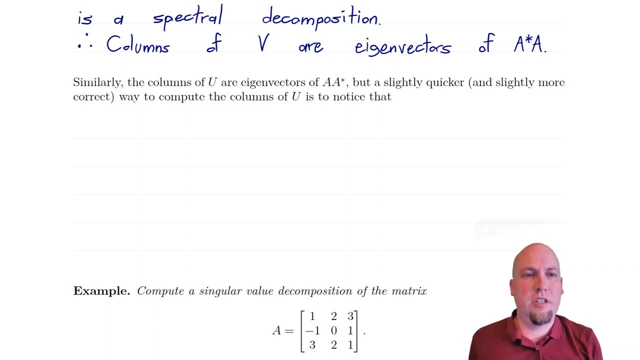 columns of u. okay. so a star a that gives you v a, a star that gives you u- okay. but you have to be a little bit careful here, because when you construct the singular value decomposition, you need the eigenvectors to sort of match up. okay, you need eigenvectors corresponding to certain eigenvalues. 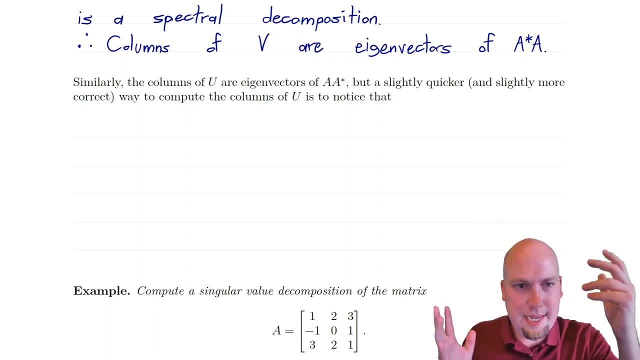 well, you need them to match up between a star, a and a, a star, so maybe an. a bit of an easier and also quicker way of computing this matrix u is instead do something like this: okay, notice that. hey, if you have a singular value, decomposition, well, i can multiply both of these. uh, multiply. 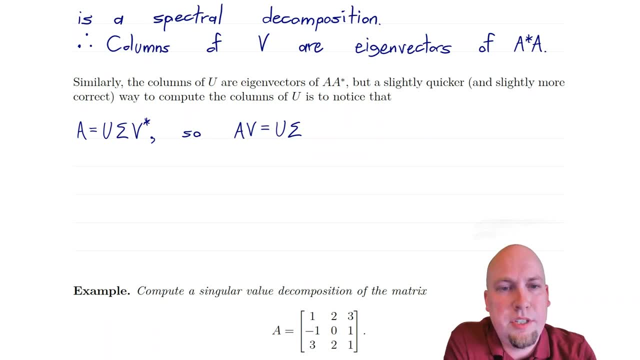 this equation on the right by v and what i'm going to get is av equals u sigma. right, then the v star v are going to cancel out. all right. and if i express this matrix multiplication in terms of the columns of v and the columns of a star a, that gives you a singular value: decomposition. 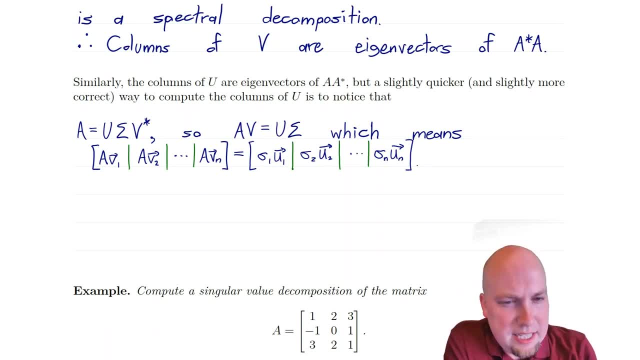 of u. what do i get? i get exactly this equation here. okay, if i do a times v, well, one way of writing that is like this: where v1 is the first column of big v and v2 is the second column of big v, and so on down the line. okay, it's just a times. each of those columns are the new columns. 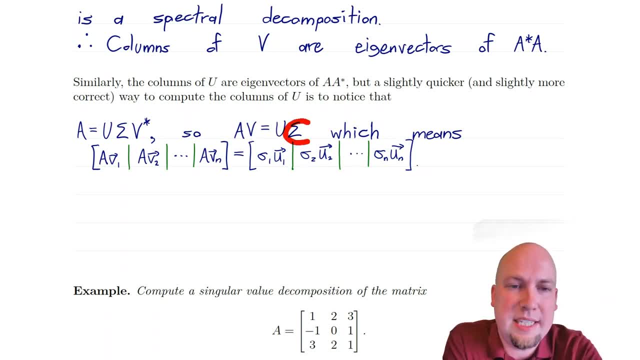 of this product on the left, okay, and similarly on the right, because sigma is diagonal. you can write this product on the right in this way: where again these u's? those are just the columns of the matrix big u? okay, so it's first sigma and then the second column of the matrix big u? okay, so it's. 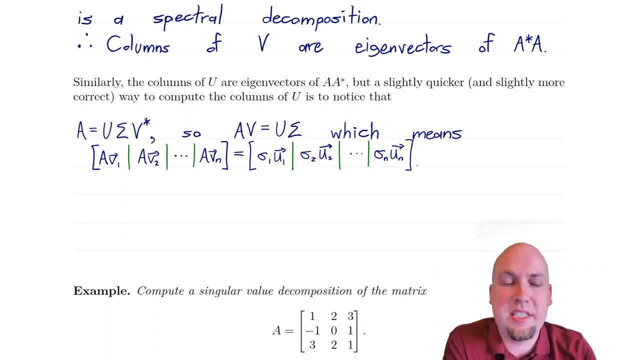 first sigma and then the second column of the matrix big u. so again the second column of the matrix big u. okay. so it's first sigma and then the second column of the matrix big u. okay. so it's first sigma and then the second column, union of all the columns of a, 0 and 2. so then whatıyorum? 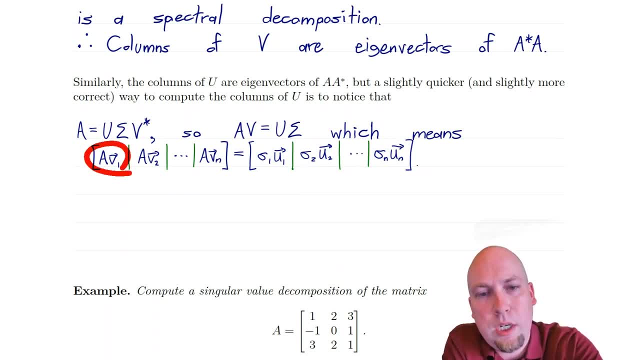 v, all of the columns of different moy by a, your, one of the columns of a dot, or did i just mention it? firstly, just go over this uh here, so also you can track this, write down theestens. so let's see a v1, 1 times second. third volume of u one up three times first. column of u four times second. 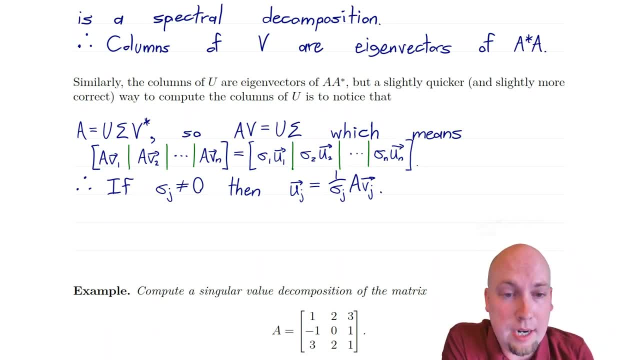 value times. second column of u. so on that line, all right. and then you just sort of set these equal of A star A. then now we can compute these columns of U as well. just rearrange the divide, the sigmas, okay. So just rearrange it so that U1,, for example, is AV1 divided by sigma 1, and U2 is AV2. 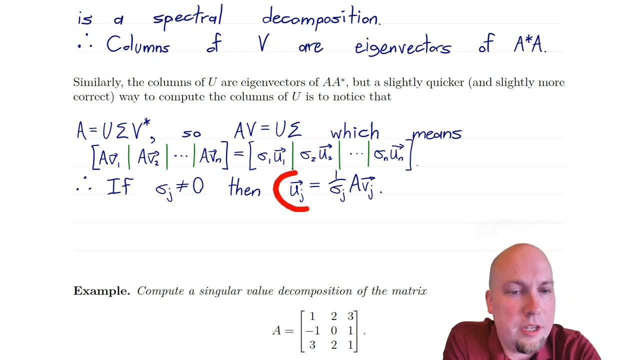 divided by sigma 2, and so on. In general, no matter what J is, UJ, equals 1 over sigma. J times AVJ. okay, So you don't need to do a second eigenvector calculation. okay, Once you do the 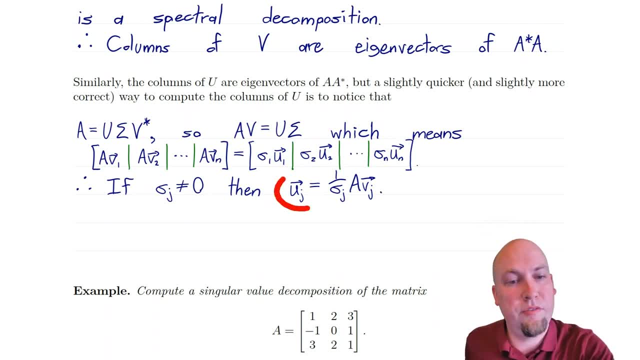 eigenvalues and eigenvectors of A star A. you can compute the columns of U, you know, just with a sort of matrix vector multiplication here. okay, You don't have to do another eigenvector calculation. However, this only works if your singular value is non-zero, because otherwise you can't do this. 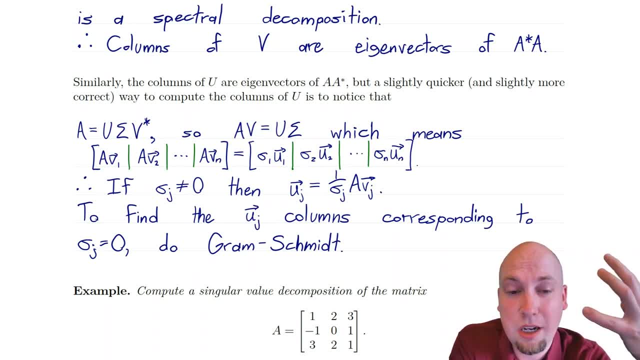 division okay, So that maybe worries us a little bit, but it turns out it's not too much of a hindrance. It turns out, if your singular values are equal to zero, you can pick that column. you know UJ to be whatever you want, as long as the matrix is still unitary, All you. 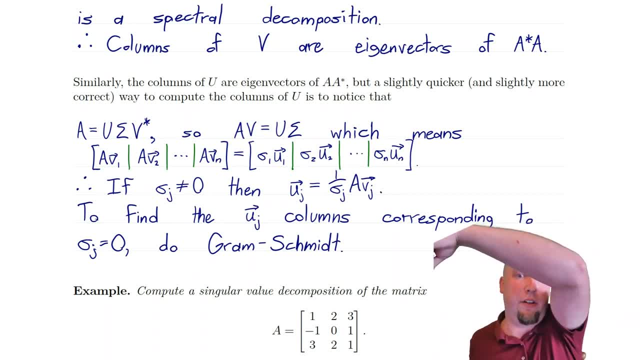 need is that it has length 1 and it's orthogonal to the other columns. okay, So, for example, you can just do Gram-Schmidt to get whatever column you want there when the singular values are equal to zero. okay, So that's a bit of a mouthful. Let's go through an example. It's not. 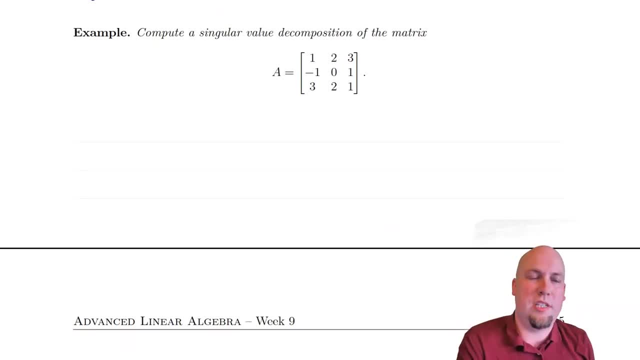 that complicated in practice. okay, It's mostly things that we've done a whole bunch of times already. all right, So let's compute a full singular value decomposition of this matrix. okay, So, step one, step one, we're going to do eigenstuff to A star A. We're going 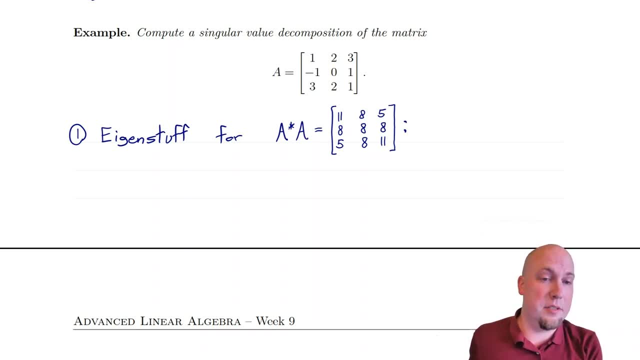 to compute eigenvalues. take square roots. that'll give us the singular values. We're going to compute eigenvectors. those will be the columns of V. All right, so eigenstuff. Again, I'm skipping over calculation here, because we know how to do eigenstuff. okay, We've done it a million times. 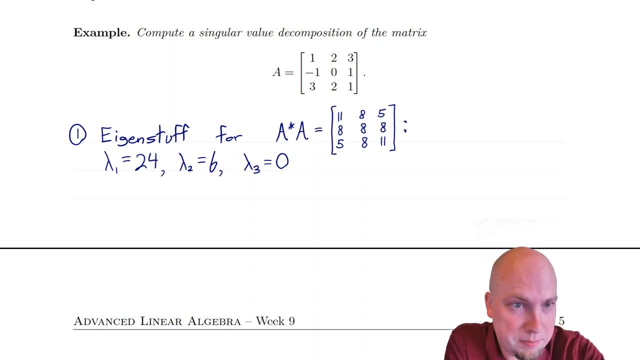 by now. So it turns out for this matrix A star A. we had to compute this, by the way. right, We computed this from this. we plugged in A star, we multiplied it by A and we got this matrix here. 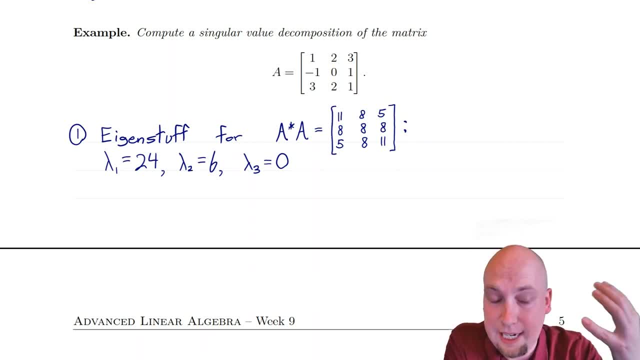 So that's a calculation. And then we compute the eigenvalues of this matrix. Again, that's calculation. We get these three eigenvalues: 24, 6, and 0. Okay, next find corresponding eigenvectors. Okay, and again, this is a calculation. 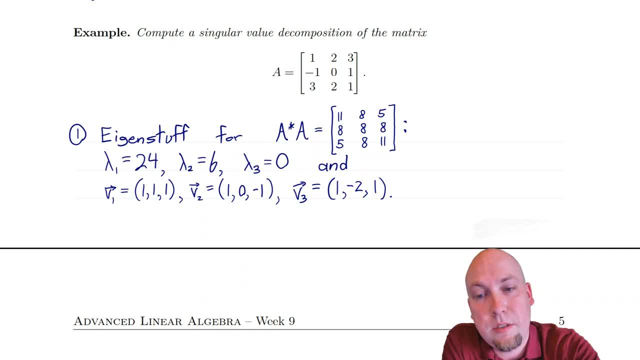 but you know how to do it. You know how to find eigenvectors. Okay so, eigenvector corresponding to lambda equals 24, it's 1, 1, 1.. Eigenvector corresponding to lambda equals 6, well, 1, 0,. 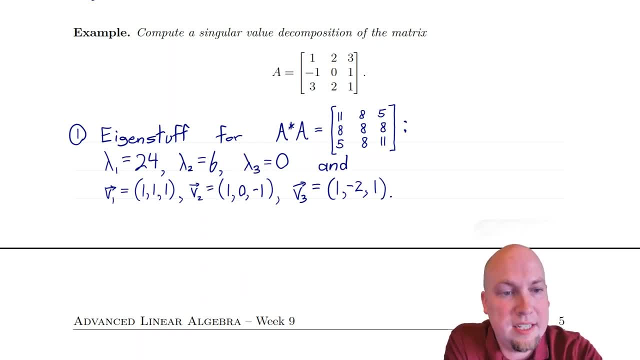 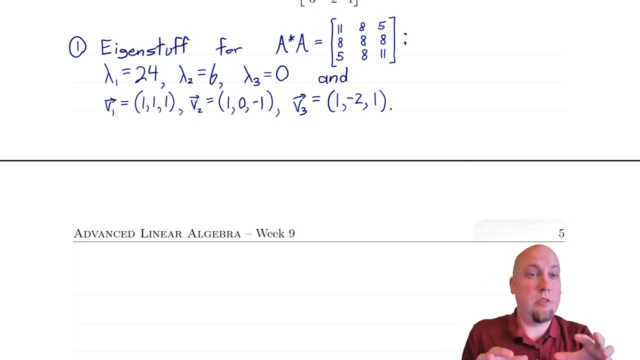 minus 1.. And eigenvector corresponding to lambda equals 0 is 1, minus 2, 1.. All right, fine and dandy. Now, once you have those pieces of information, you've actually got two of the three pieces of the singular value decomposition already, once you've done eigenstuff to A star A. 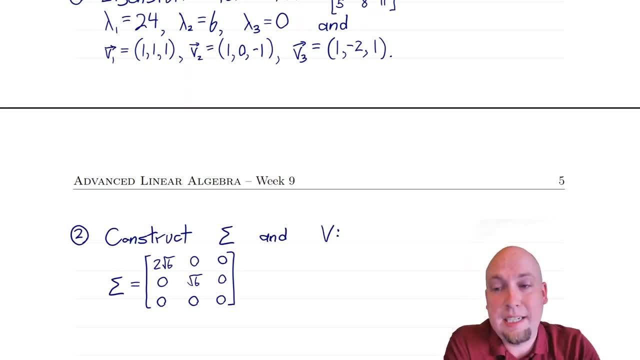 Okay, and what it is is well, now you can construct sigma and V. How do you construct sigma? You just take square roots of these eigenvalues and stick them down the diagonal. So square root 24, ah, that's 2 root 6.. So that's my largest singular value. I'm going to stick it. 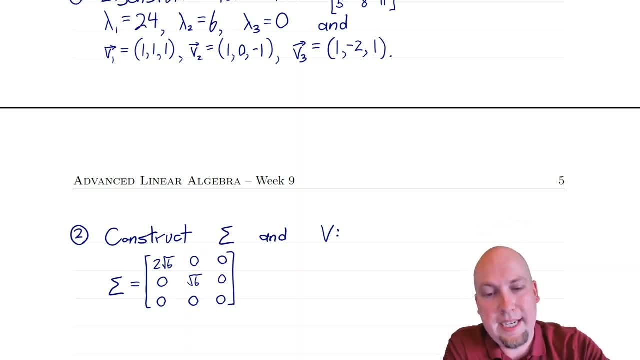 at the top left. Square root of 6 is going to be my next largest singular value. That's my next diagonal entry. Square root of 0 is my next largest singular value. That's my next diagonal entry. Okay, so that's all there is to constructing sigma, the diagonal matrix in the middle. 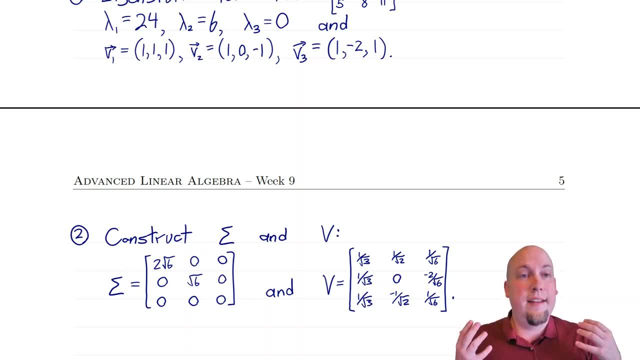 How do I construct V? Okay, it just comes from the eigenvectors of A star, A. Okay, and I've already got these here. So these are going to be the columns of V, except I have to be careful: Make sure you normalize them. Okay, in general, make sure that they form an orthonormal basis of you. 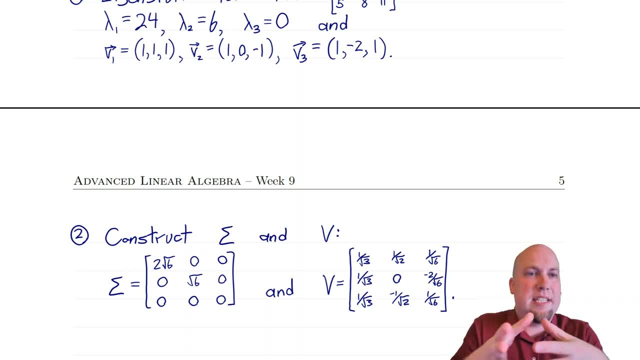 know the full n-dimensional space. Okay here, because every eigenspace is just one-dimensional, all I have to do is normalize. But if you have a two-dimensional or larger eigenspace, you might have to do Gram-Schmidt to make sure that they're orthogonal to each other as well. All right, so? 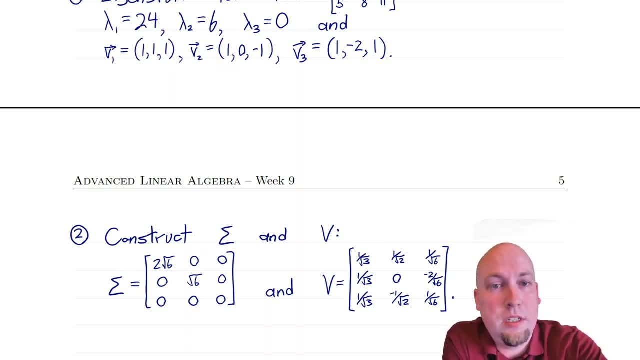 1 divided by root 3,, so that has length 1.. 1, 0, minus 1, divide by root 2,, so that has length 1. again Okay, and then 1, minus 2, 1, divide by root 6,, so that it has length or norm equal to 1. this 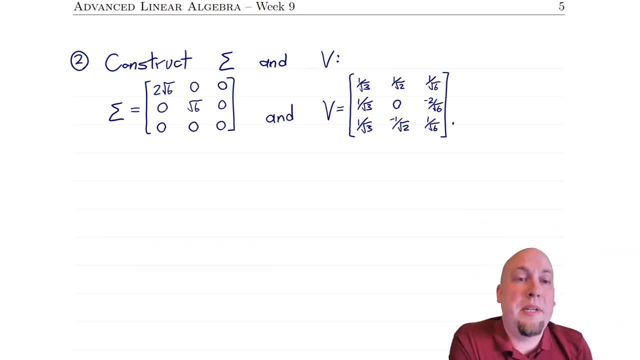 time. All right. so there's sigma and V. That's two out of the three pieces of the singular value decomposition. Next up, we just need to construct U and then we're done. Okay, the left unitary matrix: Okay. and the way you do this is as we talked about before: for every non-zero singular, 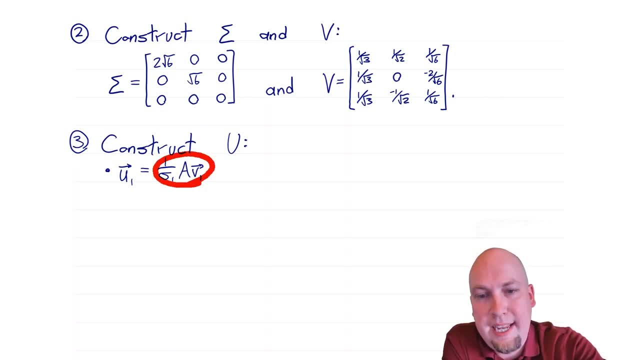 value you do 1,, 0, minus 1, divided by root 3,, so that has length 1.. 1, 0, minus 1, divided by root 2, 1 over sigma j times A, Vj. Okay, so my largest singular value is 2 root 6, so 1 over 2 root 6. 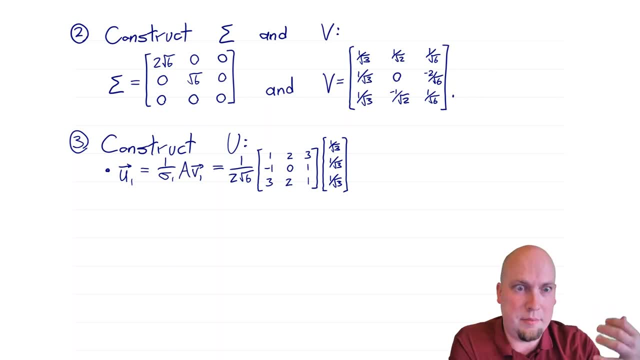 times A. So this is just copying the matrix A from the question, And then V1,. well, that's the first column of V. Okay, so you just do a matrix multiplication now and you get your answer. Okay, and after simplifying a little bit, it turns out that it's 1 over root, 2 times 1, 0, 1.. That's my 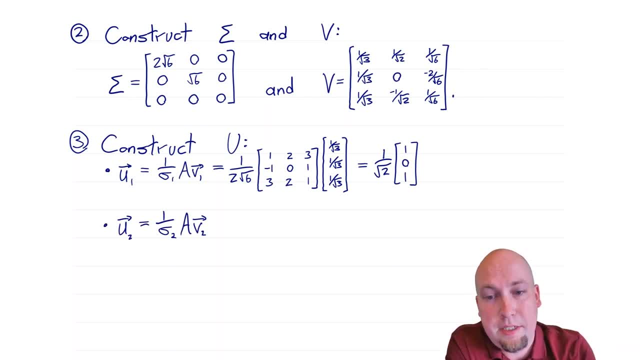 first column of U. Next up, I do 1 over sigma 2, A times V2.. Same thing, just increase the subscript. Okay. so what is sigma 2?? It's root 6, so 1 over root 6.. 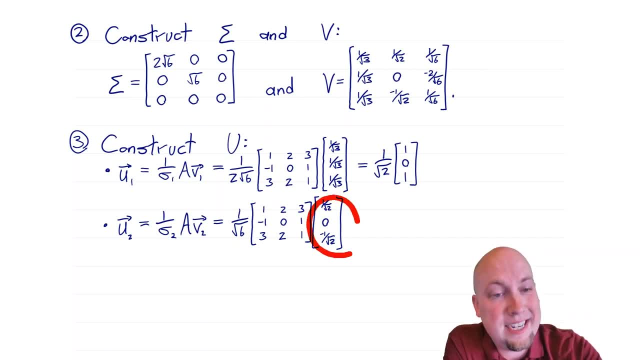 Here's the same matrix A still, and now here's the second column of V. I just copy and pasted it down there. Okay, there's the second column of V. I do my matrix multiplication. This time I'm going to. 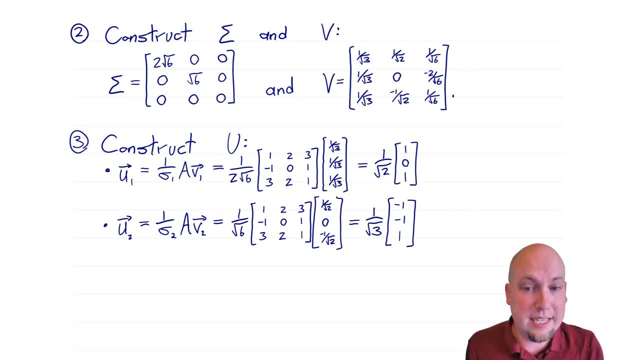 get minus 1, minus 1, 1, all divided by root 3.. Okay, so that's my second column of U, And one thing to notice here is both of these they have norm 1, and that is always going to happen as long. 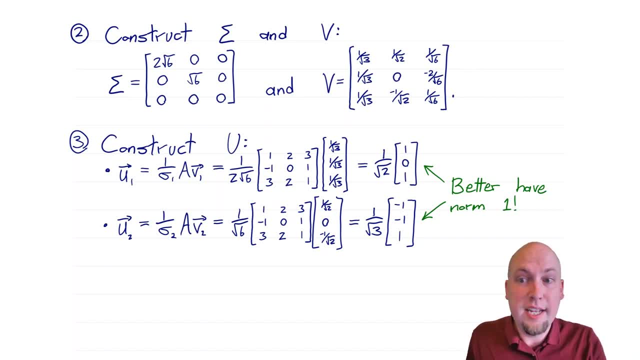 as you've done your calculations right, as long as nothing's gone haywire in your calculation, These had better have norm 1, because, well, they're going to be columns of a unitary matrix. Okay, unfortunately they do. All right, we still have one more column that we've got to construct. 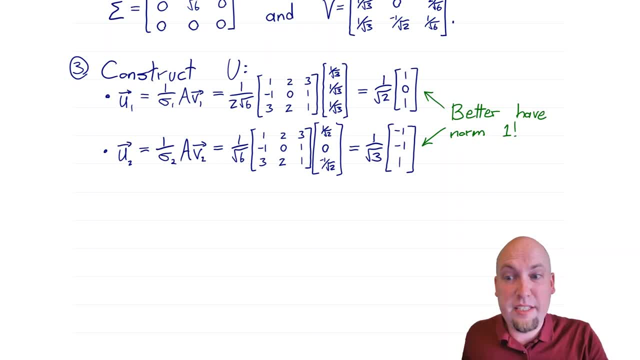 right, This is going to be a 3 by 3 unitary matrix. We need to find a third column, but uh-oh, sigma 3 equals 0.. Our third singular value equals 0.. Okay, so how do we find this third? 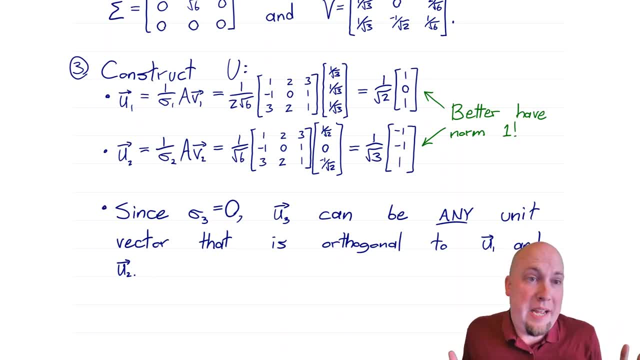 column of U. Well, it sort of doesn't matter, okay. Third column of U: it can be anything as long as the matrix is still unitary. Okay, so you need to make sure that two things happen. You need to make sure that that third column has length 1,. 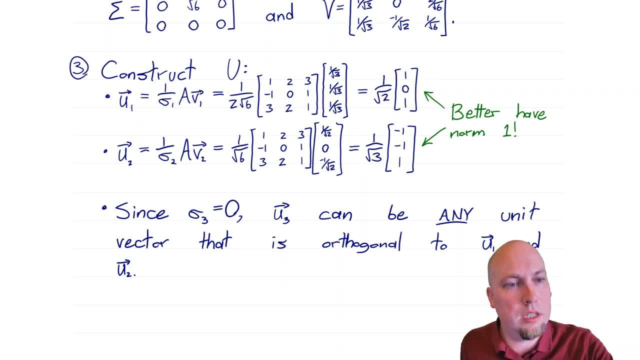 and you need to make sure that it's orthogonal to these two other columns that I already found All right. well, there are lots of ways that you can do that. We could do Gram-Schmidt procedure right. I could just pick any vector that you know when you throw it together with these two. 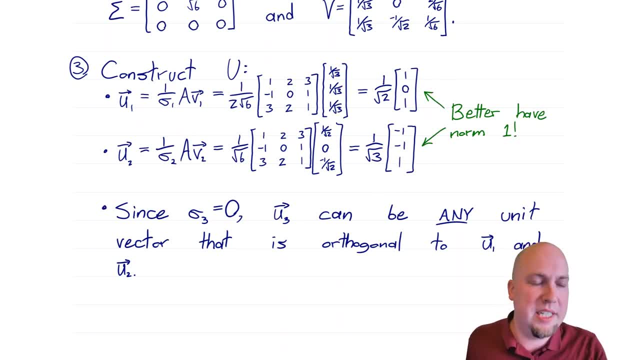 vectors makes a linearly independent set and then apply Gram-Schmidt to that set and that would give me an orthonormal basis of that. That would be one way to go. Another way to go because I'm working in three dimensions here. 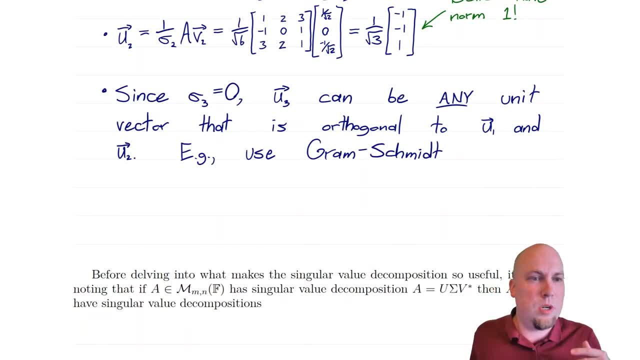 and I just want it to be orthogonal to two particular vectors. I could just use the cross product, Okay, so another way to do it in this particular case is I just take the cross product of these two vectors and when I do that, so here I just copied down, you know. 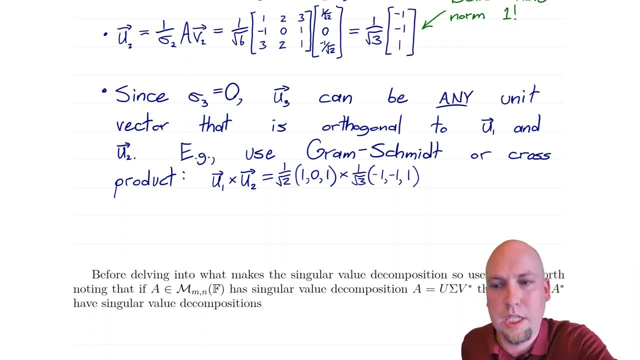 one of the vectors I found, and here I copied down the other column of U that I found. I do that cross product and I get 1 over root, 6 times the vector 1 minus 2 minus 1.. Okay, and again. 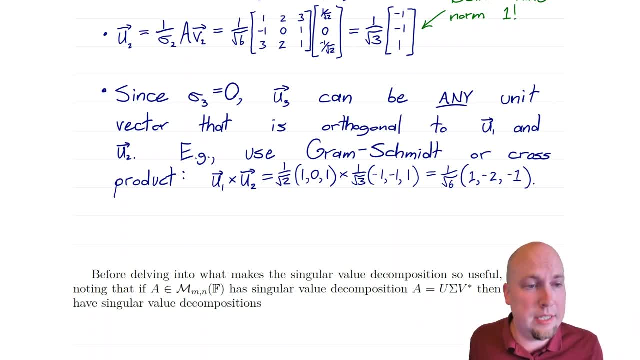 that's a very simple way to do it. So I just take the cross product of these two vectors and I just unit vector. If you've done things right, it had better be a unit vector. So that just becomes my third column of U. I know when I take the cross product of two vectors I'm going to get something. 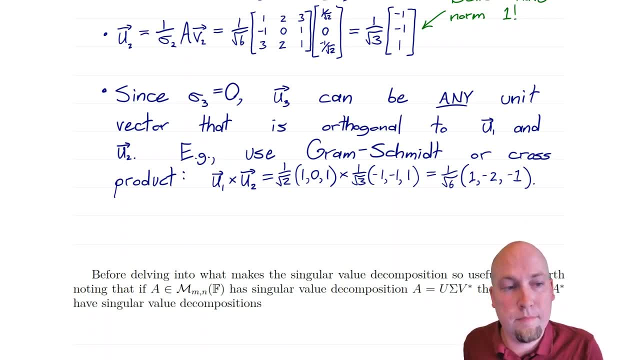 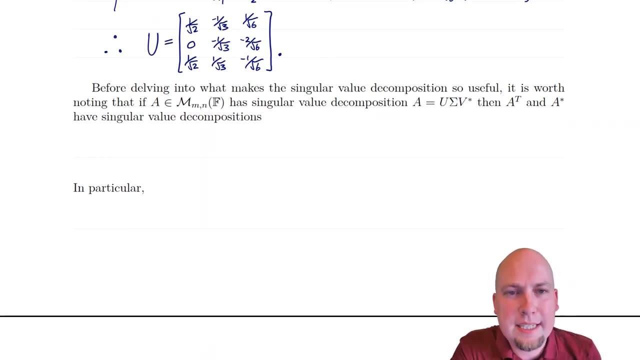 that's orthogonal to those two vectors that I started with. All right, so that's an- okay, third column of a unitary matrix U. So that's my unitary matrix. and then I'm done. That's the third piece of my singular value decomposition. so I'm done. Okay, that's all there is to it. Okay, so the last. 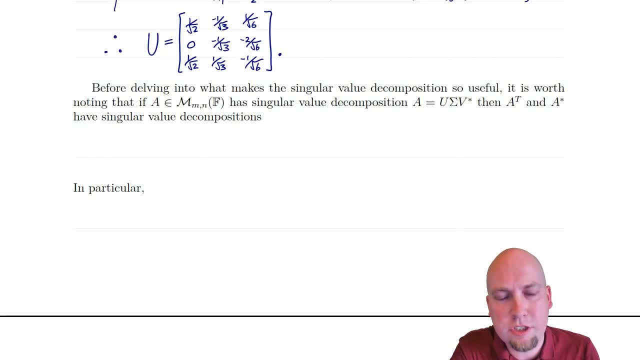 thing I want to talk about in this lecture is how the singular value decomposition changes if you take the transpose, or conjugate transpose of a matrix. Okay, so if you start off with the singular value decomposition of A, well, what's the singular value decomposition of A transpose? 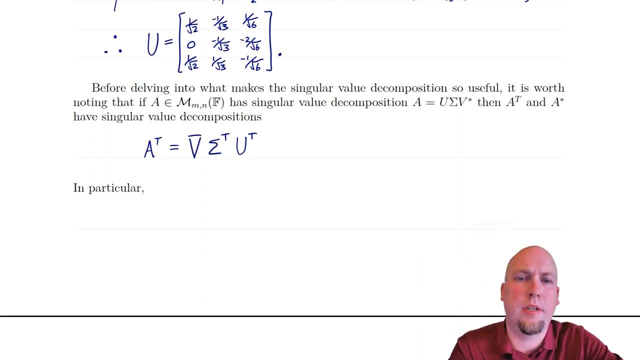 or A star look like. Okay, and this is just a straightforward calculation. For example, A transpose. well, if I transpose this product here, remember it applies the transpose to each of the matrices in the product and swaps the order of multiplication. So V star that becomes a V star. 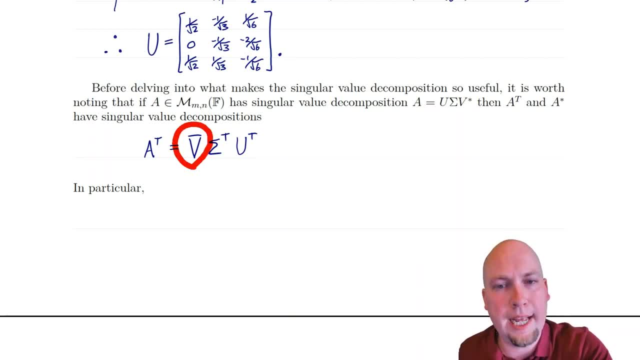 transpose all the way on the left. In other words, just a V bar. Now it just has a complex conjugate on every entry of V, but there's a V bar on every entry of V. So if I transpose this product here, 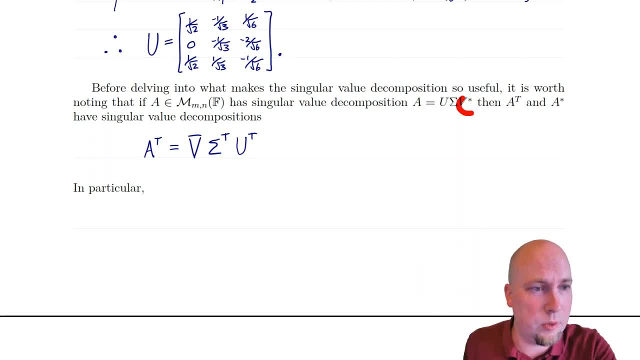 they're all in their original locations. You're not transposing anymore because it cancelled out with the star in the original V star. Okay, sigma becomes a sigma transpose and I really am writing a sigma transpose even though you know it's a diagonal matrix and the reason for that is sigma.